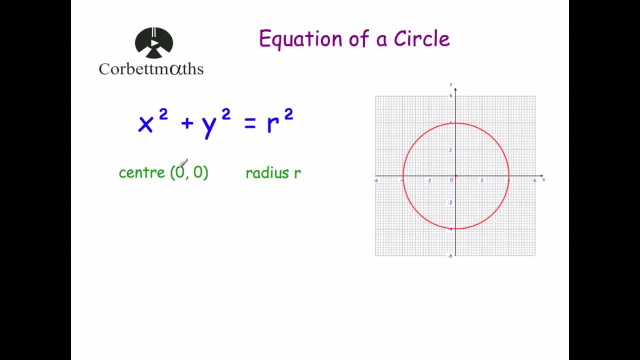 equation of. So the equation of a circle with centre as the origin 0, 0 is x squared plus y squared, equals whatever the radius is squared. So this is the format that's always in. So x squared plus y squared and equals the radius squared. Okay. so let's have a look at a question. So this: 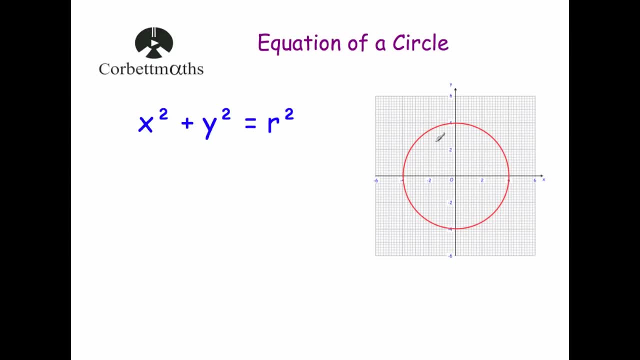 question says: find the equation of this circle. So here we've got a circle and let's we know the equation of. it's going to be x squared plus y squared, the first bit of it, because we know that the centre is the origin. Now the radius of the circle from the centre to the edge is equal to 4. 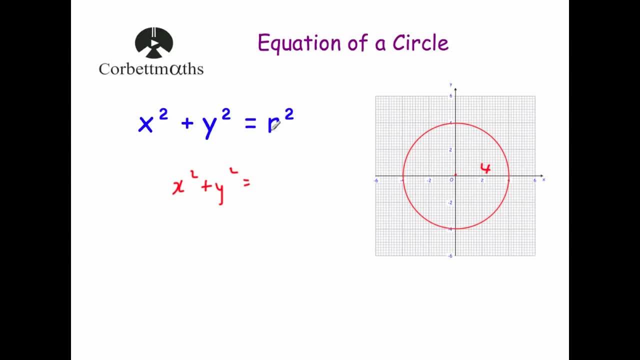 because it goes from 0 to 4.. So that means the radius is 4 and so that means it's going to be equal to whatever the radius is squared. So I'm going to write equal 16, because 4 squared is the origin of the point 0, 0, and at GCSE level they're the only circles you need to know the. 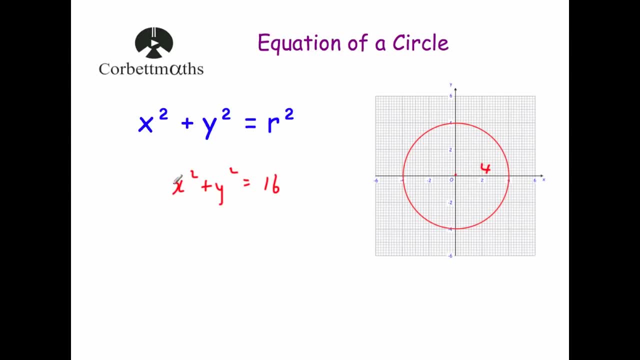 radius is 16.. And that's how I write the equation of that circle: x squared plus y squared equals the radius squared, and 4 squared is 16.. Now, sometimes in a test paper or sometimes in a question, they might not write it as x squared plus y squared equals 16. they might write it as: 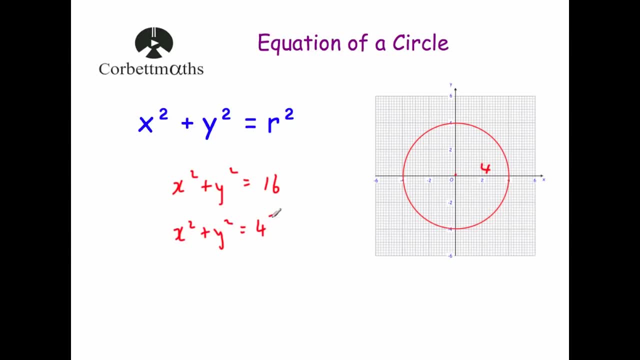 x squared plus y squared equals actually 4 squared. just actually writing down what the radius is with the squared symbol above it. Obviously, 4 squared is 16, so these two equations are identical to each other, just except for writing 16. it's written 4 squared. 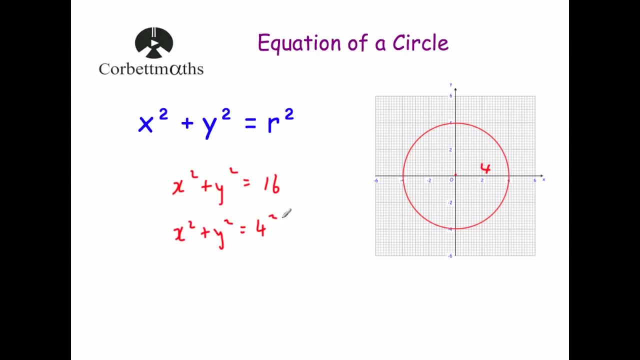 So just note that sometimes in a question you might see the equation of a circle in this format, and I like to square whatever the radius is and put it equal to that number, just because it's a habit that I've got. Okay, so here we've got a question that says: write down the equation of 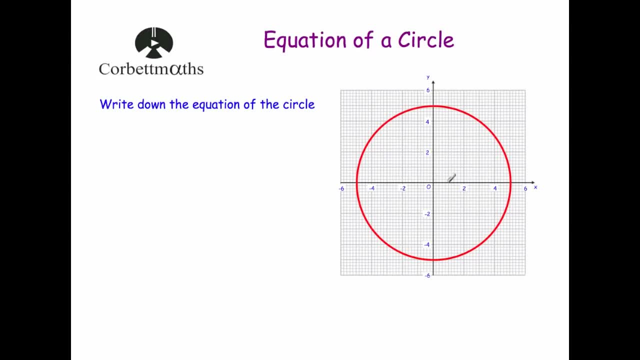 this circle. So we've got a circle and the, the radius of it, from the centre to the edge, is equal to 5.. So it's going to be equal to 5 squared and the first bit, because the centre is the origin, is going to be x squared plus y squared. 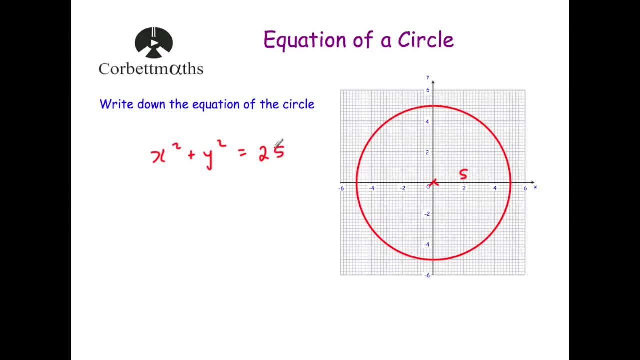 And it's equal to the radius squared. 5 squared is 25 and that's it. so that's the equation of this circle. As I've said, you could write x squared plus y squared equals 5 squared if you wanted to, but it's really up to you. Okay, next one. the next question says: draw the circle x squared plus y. 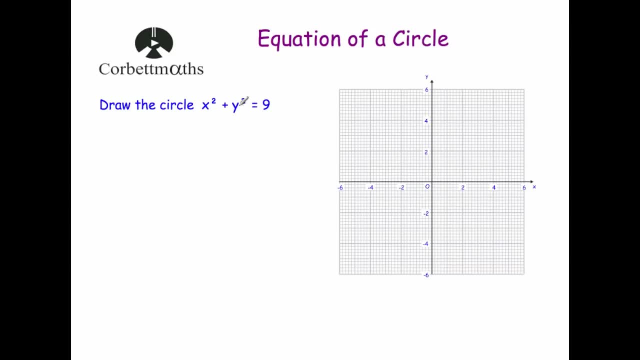 squared equals 9.. Now, at GCSE level it's going to have the centre of the origin and because it's just x squared plus y squared, we can see it's the origin. Now the radius of it. well, we've got equals 9. so what we're going to do is we're going to square root the 9. Square root of 9 is: 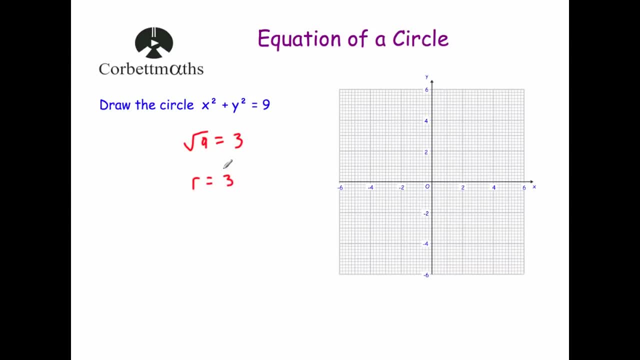 equal to 3. so we know the radius of the circle is equal to 3.. So what you would do is you would get the point of your compass, put it on the origin, you put the pencil on 3 and you draw a circle and you just be. you're just be very careful whenever you're drawing it. you draw a nice circle with your. 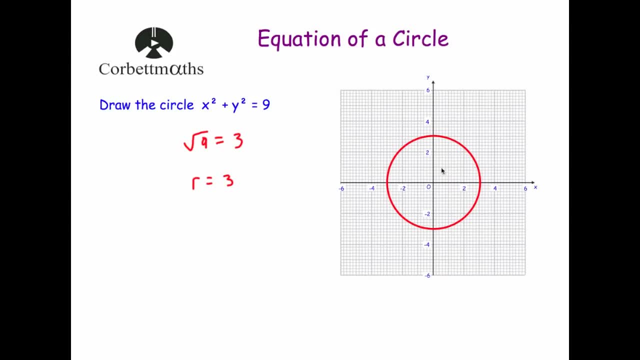 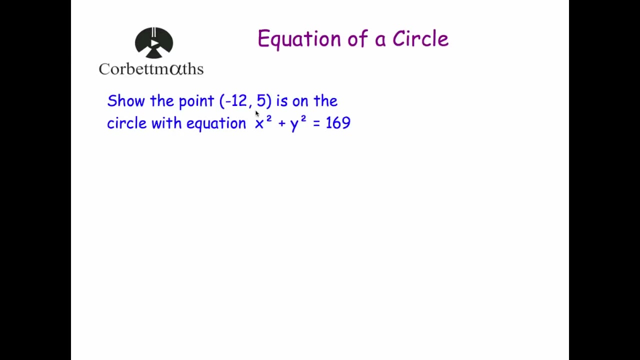 compass and it should look something like this Centre, as the origin goes through 3, 3 minus 3 minus 3 and a nice perfect circle. and use your compass when doing that. try to avoid just drawing it three hand. Okay, next question Question is asked to show the point minus 12. 5 is on the is on the circle with equation x squared. 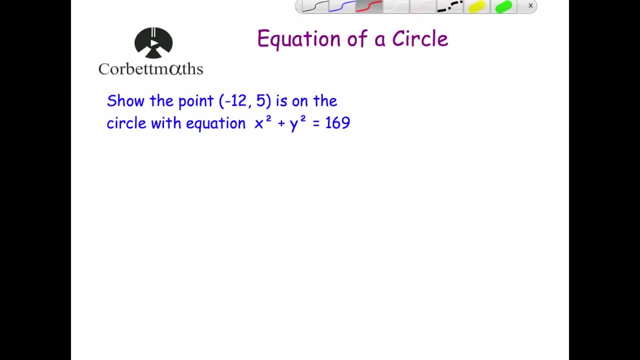 plus y squared equals 169.. So we're trying to show a point is on the circle. So what we're going to do is we're just going to know that a coordinate is in the format x and y, so the x is equal to minus. 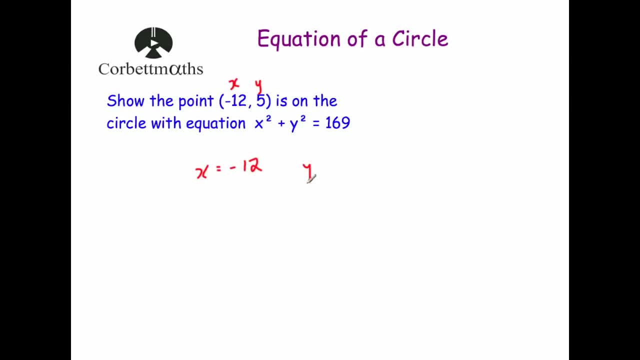 12, the y is equal to 5 and we're just going to substitute those or plug them into the formula. So the formula is: x squared plus y squared equals 169.. So it's going to be minus 12 squared. Now be very careful: if you're using a calculator for this, be very careful to make sure. 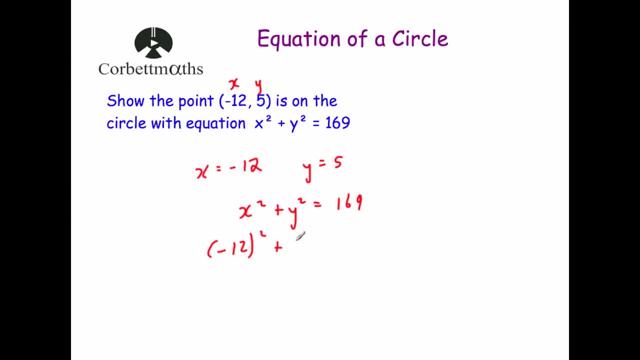 you're putting the minus 12 in brackets, plus 5 squared, and that equals, hopefully, 169.. Well, minus 12 times minus 12 is 144.. 5 squared is equal to 25 and, again, hopefully, that equals 169.. Adding these together, it was just 169 equals 169.. So, yes, it is a point on the circle: minus 12, 5 is. 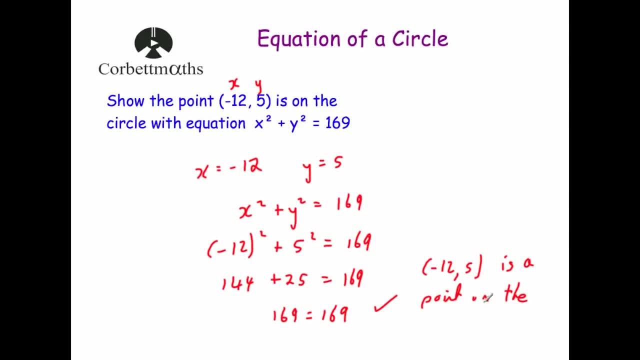 a point on the circle and that's it. So if you want to show the points on a circle, you just put in the x value and the y value into the equation of a circle and it should work out for you. If it doesn't equate, then it's either not on the circle or you've maybe made a mistake with the minus sign. 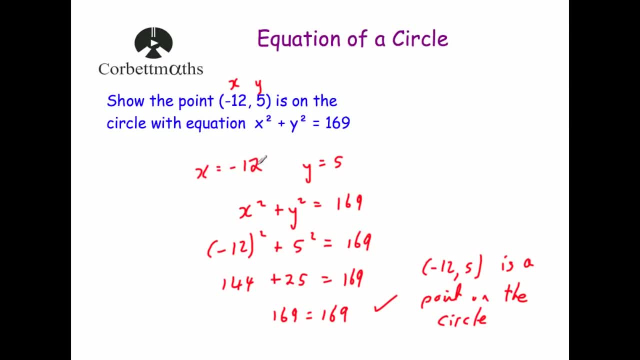 and squaring. Just be very careful, as I said, plugging into the calculator. Okay, our second last equation, our second last example. Find the equation of the circle drawn. So here we've got a circle. Now the difference between this one and the other ones are they haven't labeled the axes. 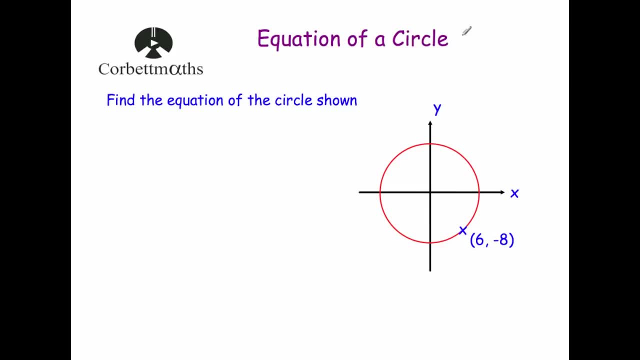 and before I could just look and see what the radius of the circle was. but here, actually, what we're going to need to do is find the radius of the circle. So we're going to draw a line from the origin to the point and what we need to do is find the length of that line. Now, what we're 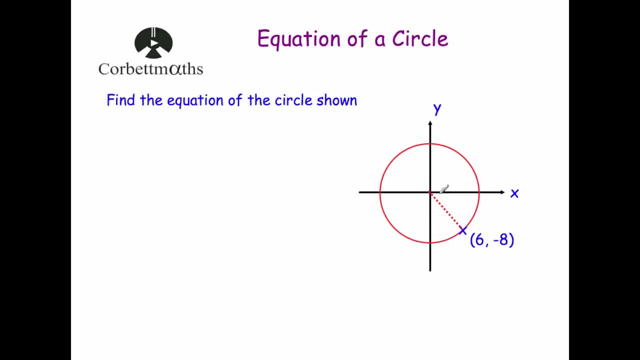 going to do is we're going to turn it into a right angle triangle, because I know this coordinate is 6 along the corridor. The x value is 6, so it's 6 along, so it's 6 along here. so that's the point. 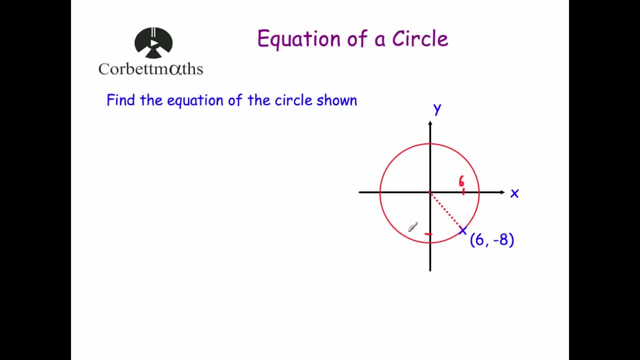 6, so it's 6 along there And it's minus 8. so we know it's 8 down here. So this is a right angle triangle there. We know that this value is 6, we know this value is 8 and we can use Pythagoras' theorem to work out the length of. 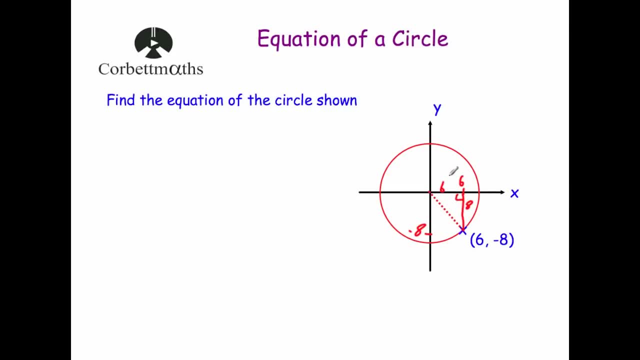 the hypotenuse and the length of the hypotenuse will be the radius of the circle. So if we label them- a shorter side, b next smallest and c being the largest, a squared plus b squared equals c squared, So the two short sides. so it's going to be 6 squared plus 8 squared equals the hypotenuse. 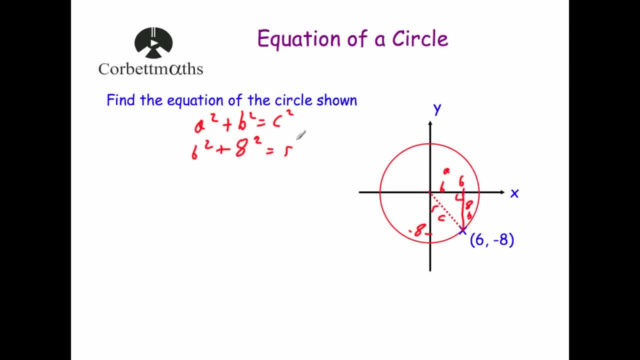 c. I'm going to call r actually for the radius squared. so 6 squared is equal to 36.. 8 squared is equal to 64, and that equals the radius squared. Adding them together gives you 100 equals r squared. and now at this point, obviously r could be plus or minus 10, but given that this is the 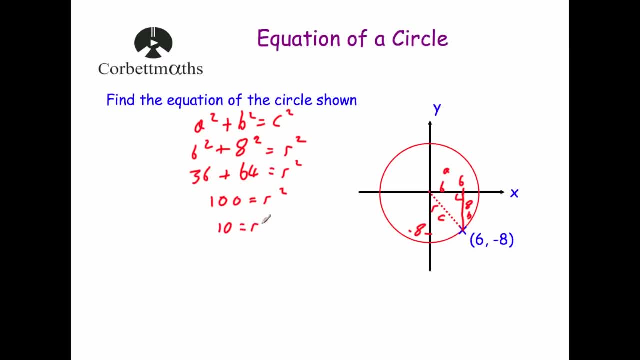 length of a line. we're just going to square it with both sides and get r equals 10.. Just be careful whenever you get equations such as x squared equals a positive value, because it could sometimes be plus or minus 10. But in this situation it could just be a positive value. So we've got: the radius here is equal to 10.. 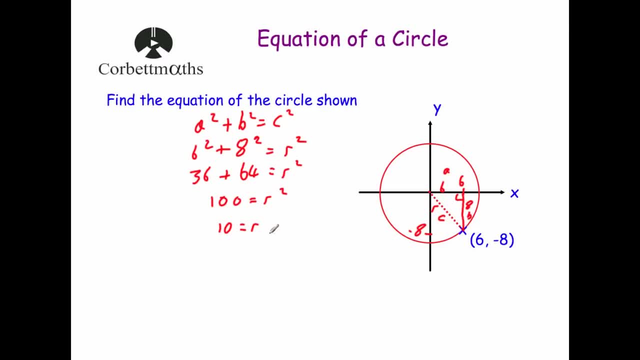 Now, those of you that know your right angle triangles, you'll know that 3, 4, 5 is what we call a Pythagorean triplet, and so we double the 3, 4, 5, we get 6, 8, 10. so that I knew the radius was.